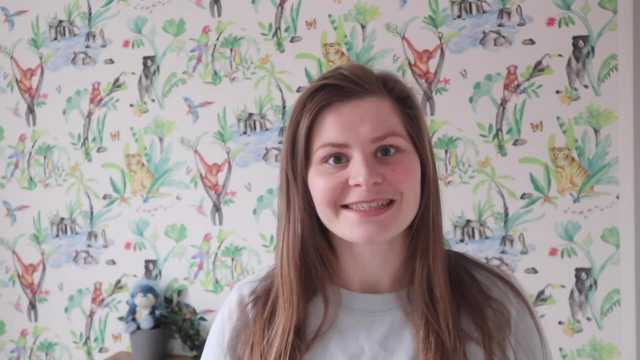 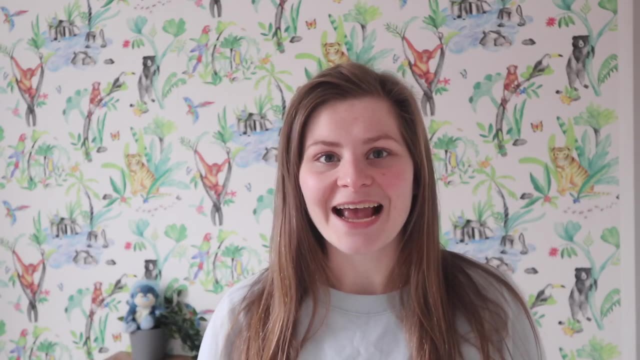 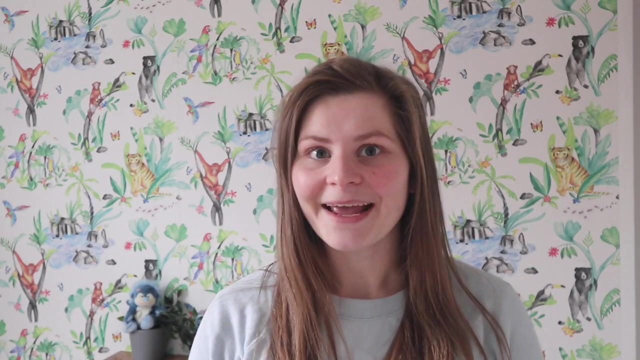 I'm going to tell you a little bit about each of the animals and I want you to see if you can guess which animal I'm talking about. I'm an unusual species because I have a bright red face. I like to eat fruit, particularly bananas, and I swing high up in the trees. 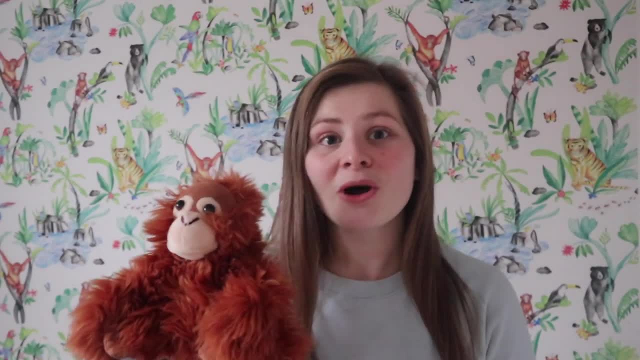 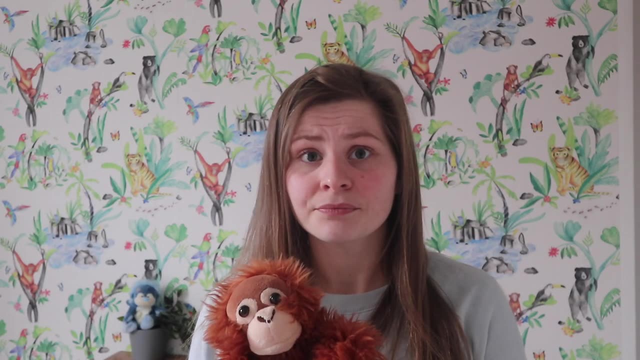 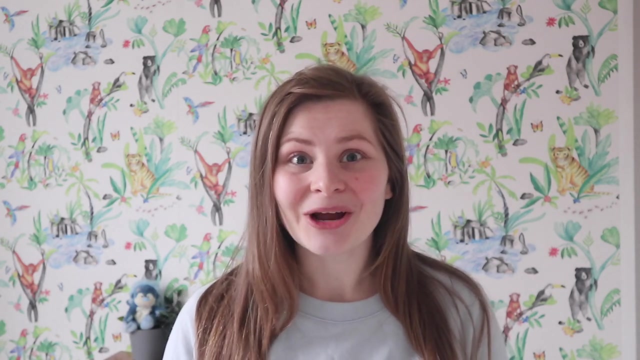 What am I? Can you guess? I'm a Wakari monkey. I'm endangered because of deforestation and hunting. The next animal also lives in the trees, But they move really, really slowly. I eat leaves, bugs and twigs. 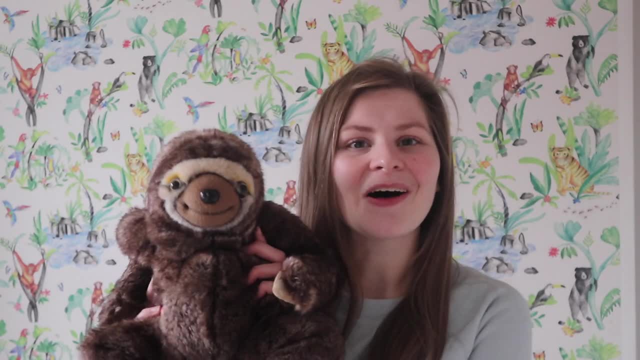 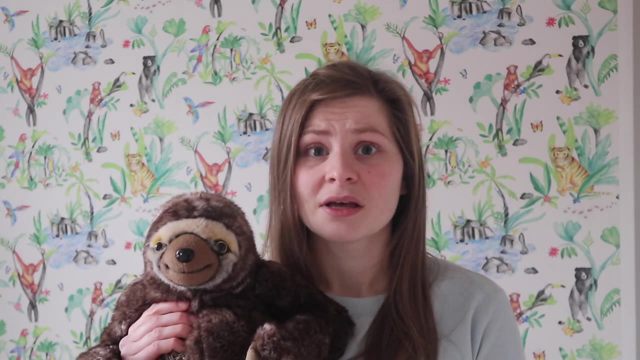 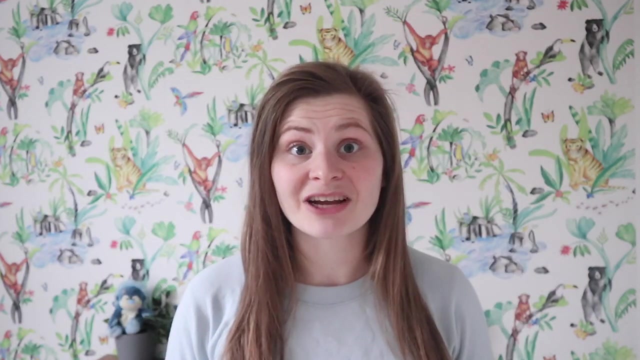 Can you guess what I am? I'm a sloth. Sloths are endangered because people are cutting down the trees that they live in. That's called deforestation. The last animal giving you a big clue here I am South America's largest. 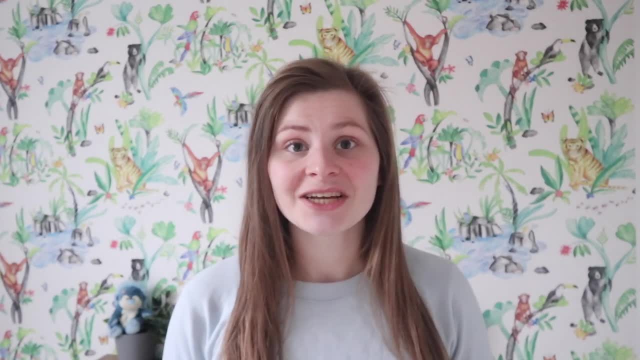 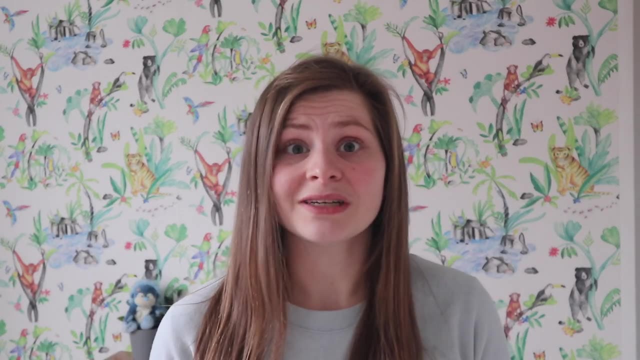 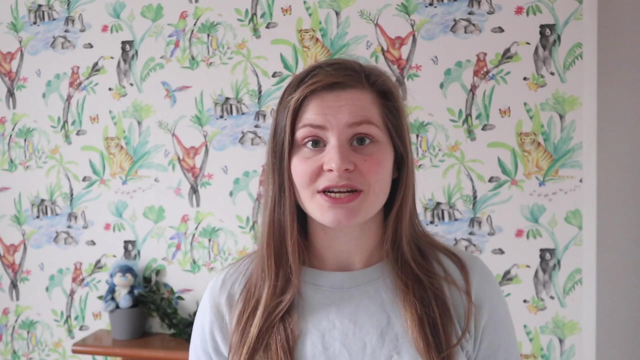 cat. I like to eat fish, deer, turtles and tapir. One of the reasons why I'm endangered is because of deforestation. Did you guess what I am? I'm a jaguar. So now you know a little bit about deforestation and the animals that you can find in the Amazon rainforest. 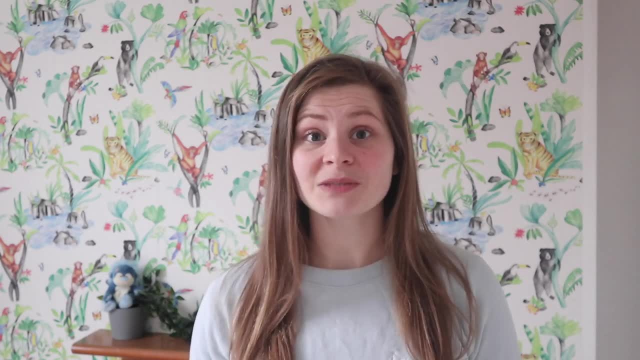 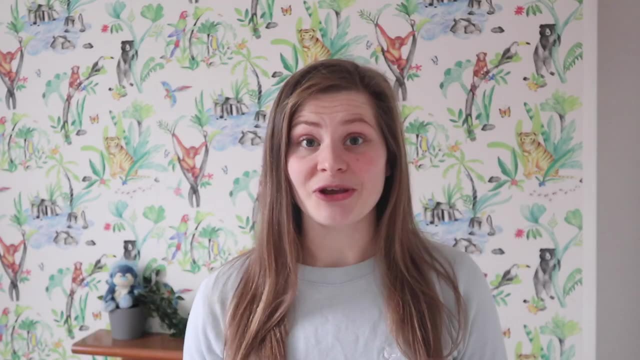 There are so many more animals, though, But the three that we've just spoken about are going to be the three that you're going to pick from to create a fact file on today, And I'm now going to show you how you're going to create that fact file. 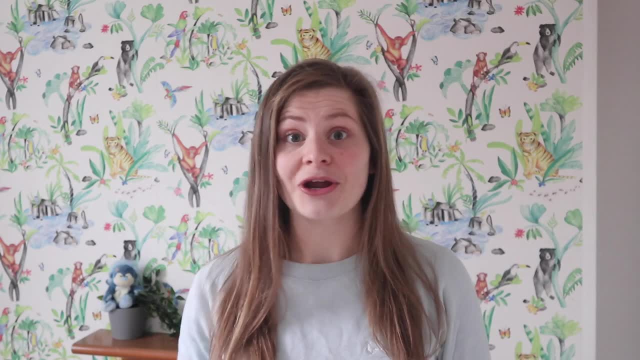 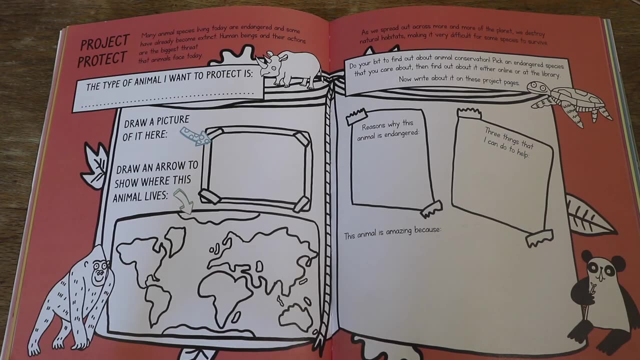 So have a think which animal you're going to choose. You can only pick one. So, boys and girls, you should have a sheet that's printed out Like this. If you haven't yet, then you can print this out after the video has finished. 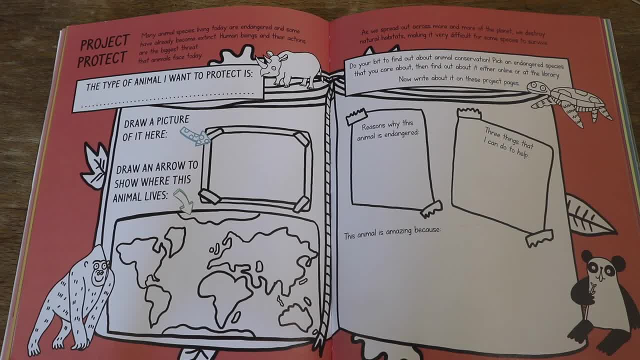 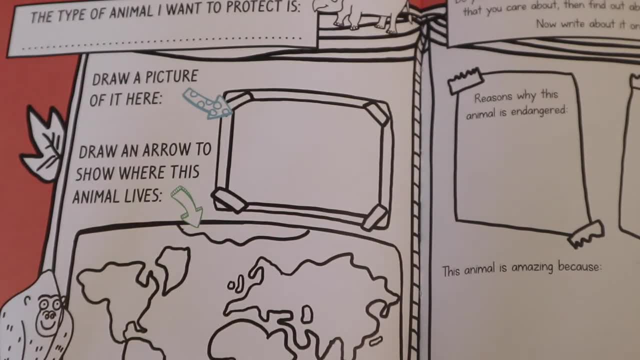 I just want to explain a little bit about what I'm expecting you to write for this. First of all, you're going to need to tell me what your animal is. You're going to list the animal there out of the three options that I have given you. 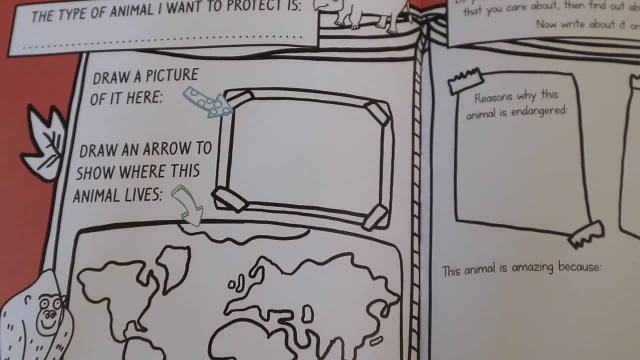 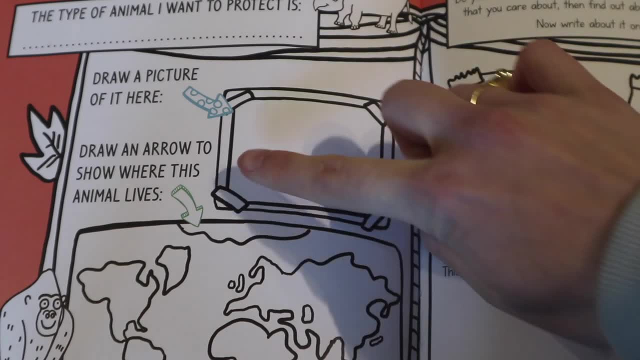 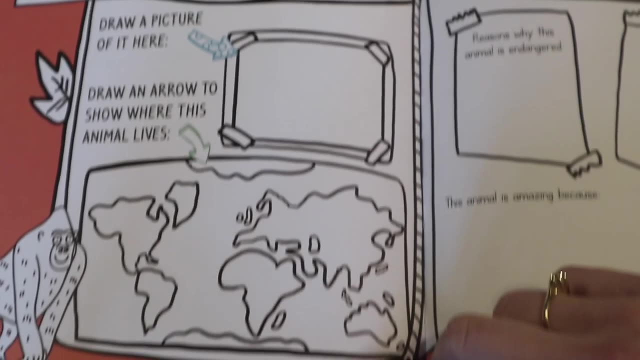 Draw a picture of it here Now. I'm not expecting you to have this drawing Amazing, Because this is an art activity, So don't spend all your time trying to get that drawing done. It's going to be imperfect. Okay, Draw a quick picture of it and move on. 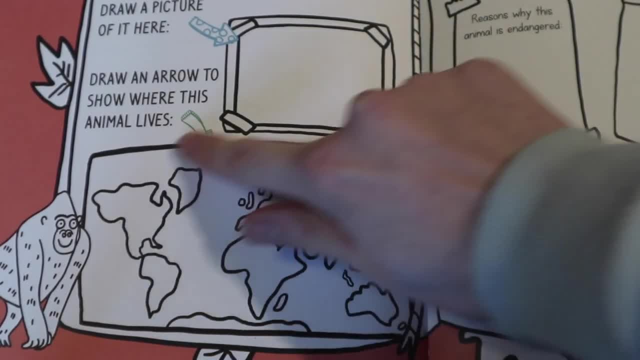 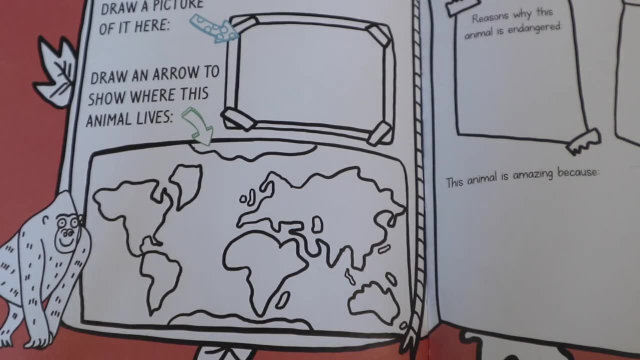 Draw an arrow to show where this animal lives. Well, you're going to need to look at this map and tell me where your animal lives on this map. You might need to look at a real map. to help you for this, I'm going to say you can use a colouring pencil to colour in the continent or country where your animal lives. 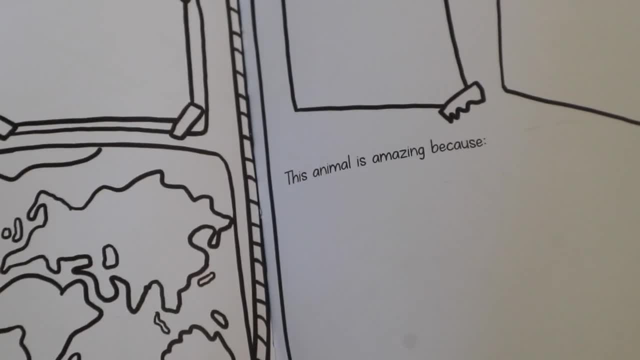 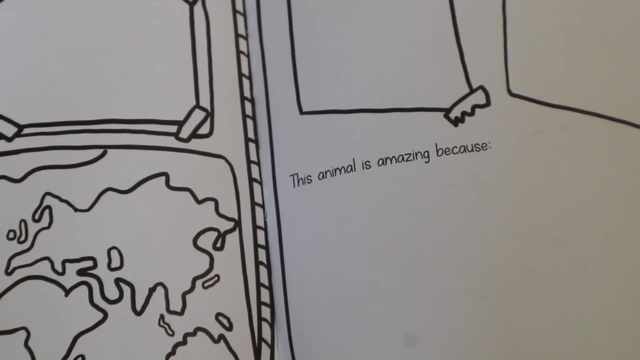 For this example, I'm going to use a colouring pencil. For this example, I'm going to use a colouring pencil. animal is amazing because I'd like you to put any facts that you can think of for your animal, and these facts can be found on the fact files that I created for your animal, As you can see. 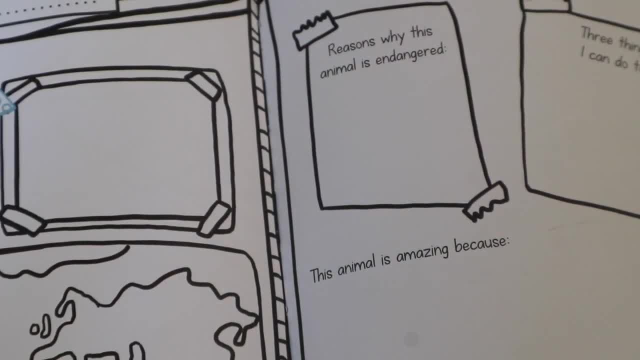 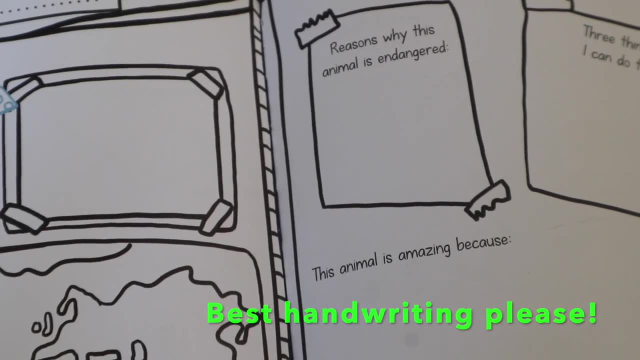 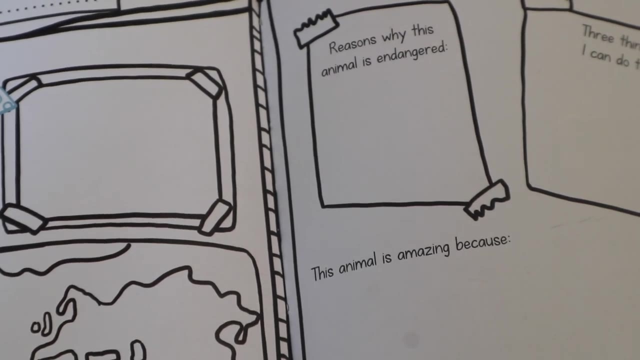 the boxes for this activity are very small, so I'm not expecting you to write a lot. I would like you to have best handwriting, making sure that you've got capital letters and full stops and double check any spellings that you're unsure about. Okay, so you can either do that in a 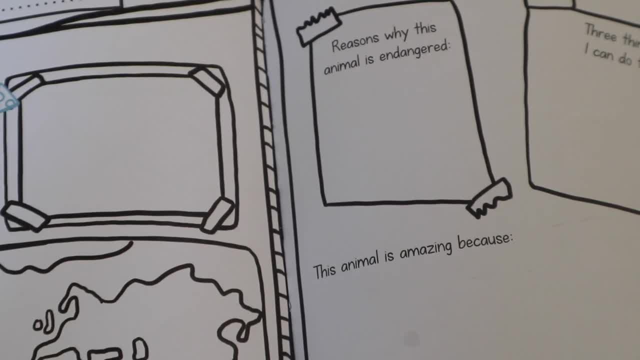 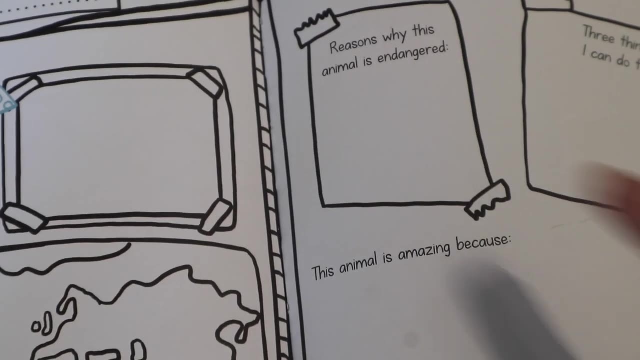 dictionary or checking the sheets that I have completed and resources that I've given you, to see if that word is on any of those that you can copy from. So I'm happy with you to do lists for this one, but what I am expecting is that you have neat handwriting The reasons for why the 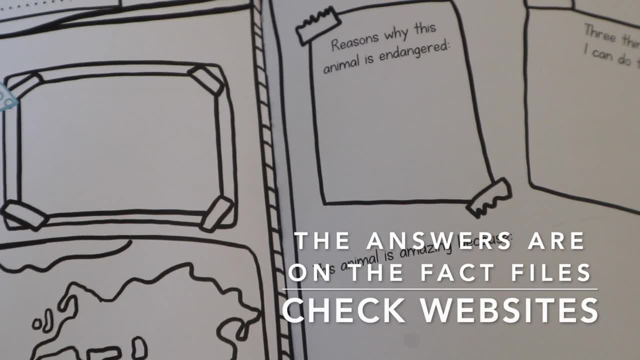 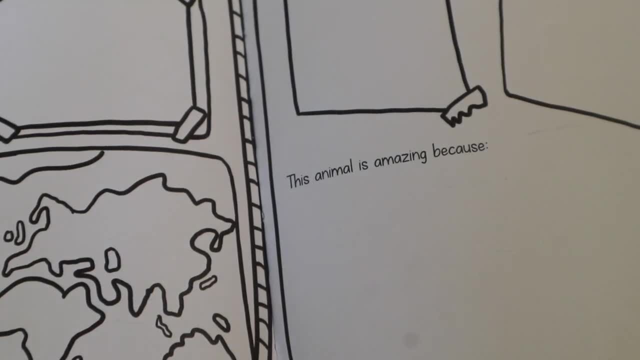 animal is endangered are the following. First of all, it's important to know that the animal is endangered. You'll be able to find these on the fact file that I created for you, but also in the website links that I have provided you with that you can go and research the animal for yourself. 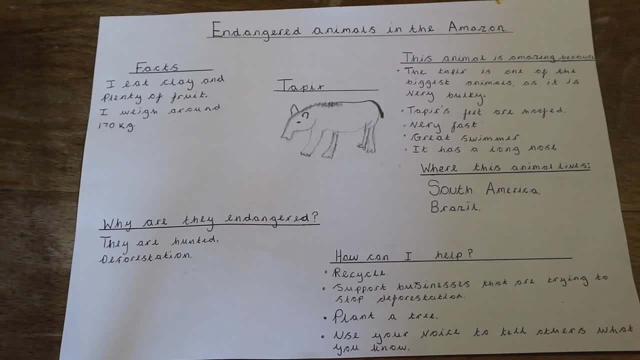 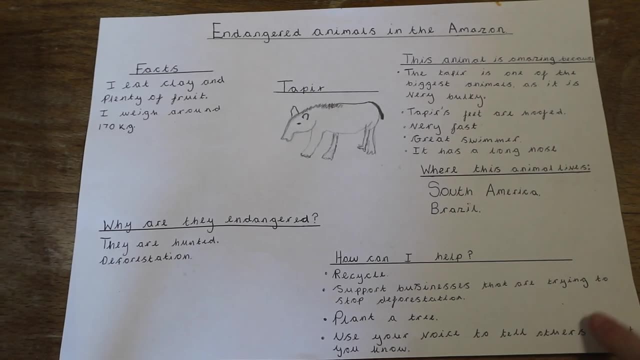 I have created a waggle for those of you that cannot print that sheet off, and this will show you exactly how I'd like it to look if you are to complete it on plain paper. But boys and girls listening that are going to print out the sheet, this is an excellent opportunity for you to now. 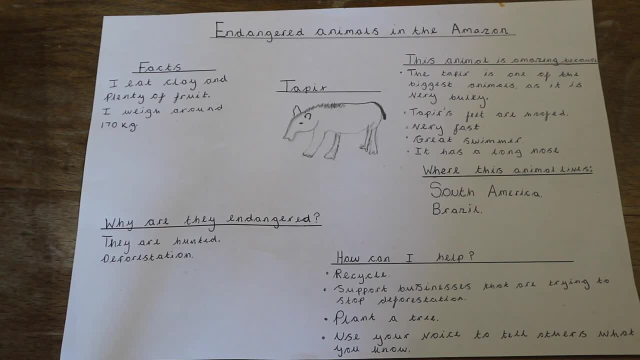 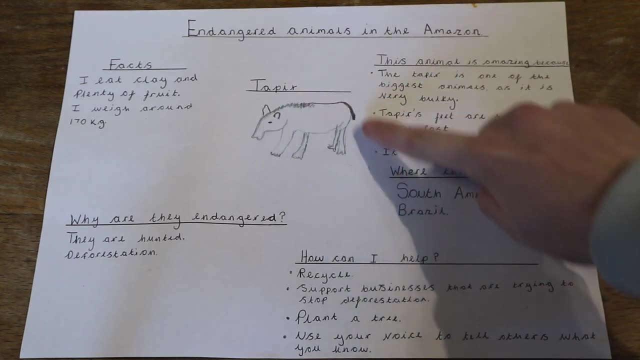 listen to the kind of things I'm expecting you to read. So if you're interested in reading this sheet, you can do that by clicking on the link in the description box below and you'll be able to see what I've written in the sheet. I've also used a ruler to underline that, and I've done that for. 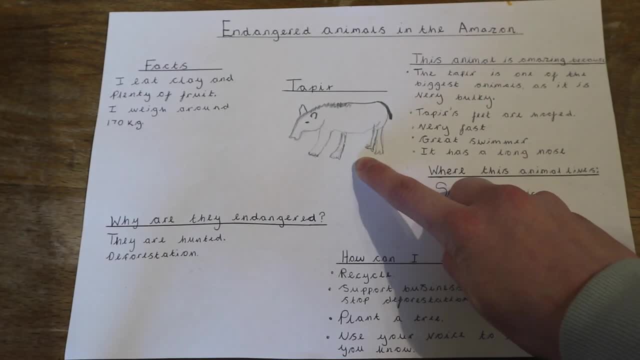 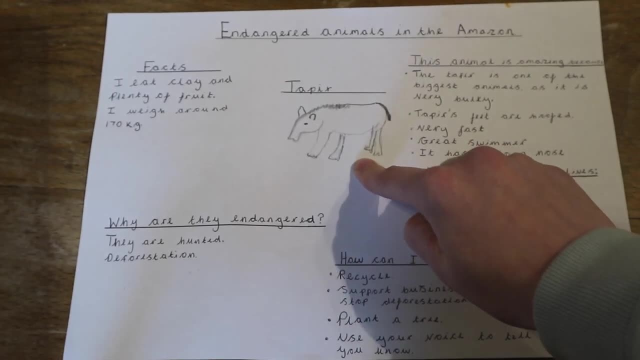 all of my subheadings. I'd also like to mention that my drawing only took me two minutes and even though it's terrible, it doesn't matter because it's not about what my drawing looks like. So don't worry if you're not happy with your drawing, because I'm not happy with mine. 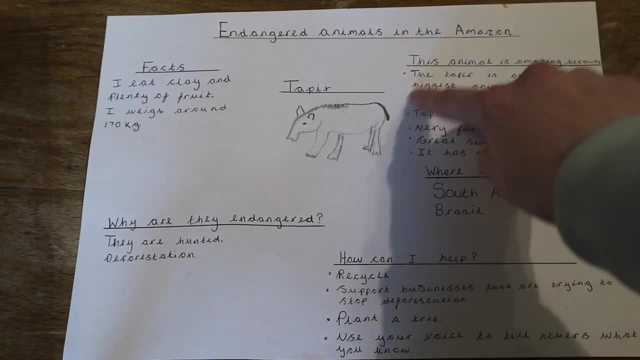 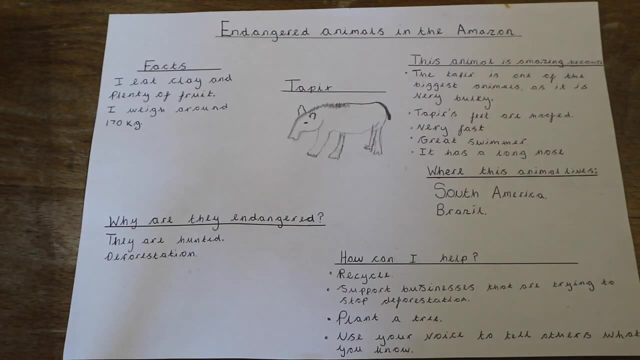 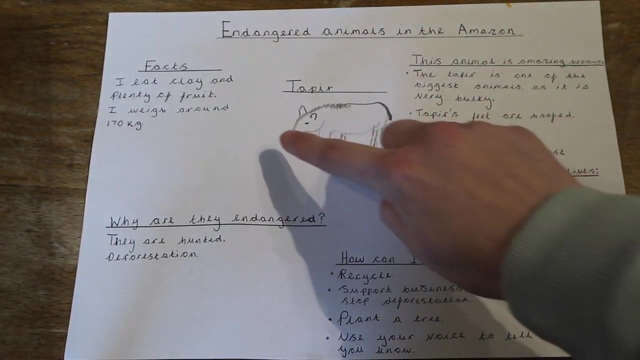 This animal is amazing because, well, I've written a few facts about this animal here and I've also added facts here just because there was enough space for me to add something else. So these two are the same. They're both facts about my animal. I've done a title. 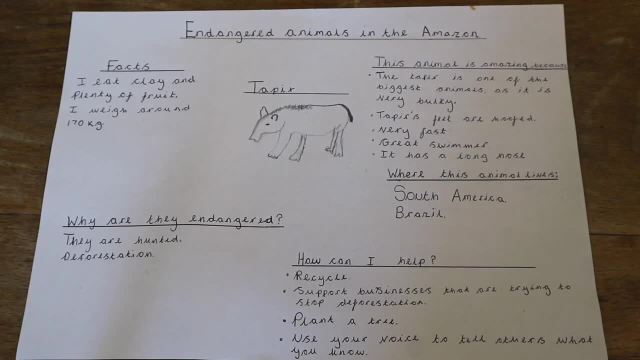 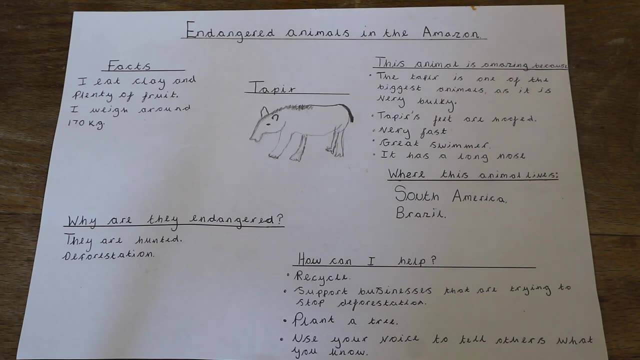 and then I've got a number of subheadings that I'd like you to include in your work. So, just like the sheet that I have attached, the sheet asks a couple of questions. What can I do to help? It also asks you to tell me on the map where the animal lives. I'm not going to expect you to draw. 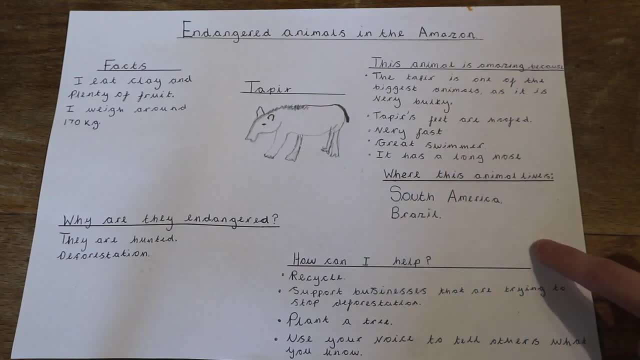 a map here That might be a little bit difficult. If you want to have a go at that and challenge yourself and draw South America and Brazil and look, locate Brazil on South America, I'd be very impressed by that, but I'm not going to expect you to do that. 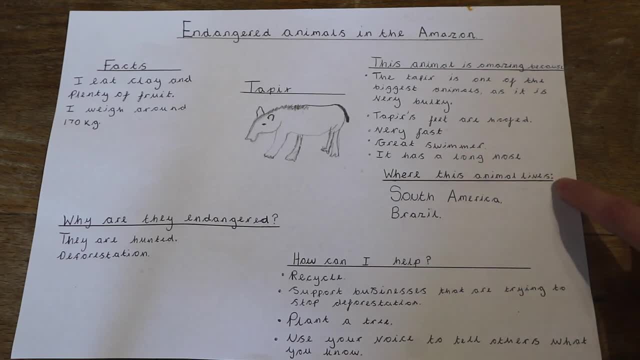 So what I've done here is where this animal lives, is my subtitle, and I've told you where I found that information out. Okay, so each of these subheadings are questions that were asked on that sheet. This is exactly how I would like it to be laid out. I'd like you to use subheadings. underline those subheadings. 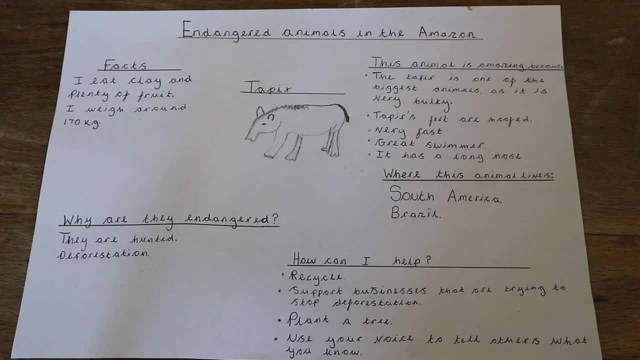 and also very important, that you have capital letters and full stops. I'm not expecting you to write sentences, just enough so that it makes sense what you mean. Okay, so for here I have written a sentence. my sentence starts with the capital letter and ends with a full stop. I've capitalised Amazon. 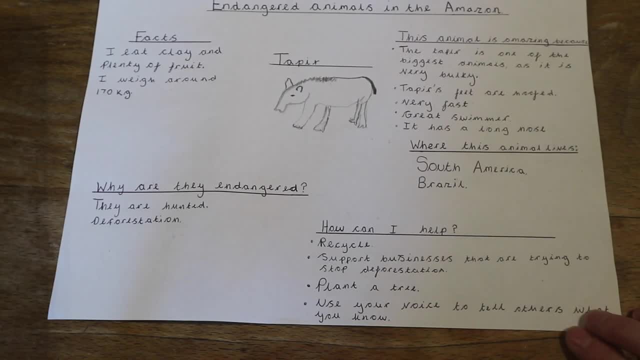 because that's a place. I've given four reasons why I can help. I only asked you to write one a month. There are a number of reasons why I can help. I only asked you to write one a month. I only asked you to write one a month. 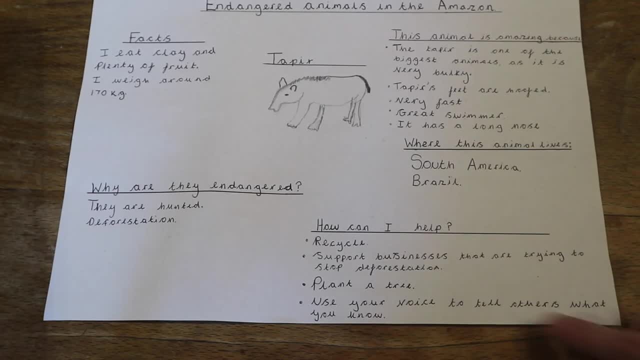 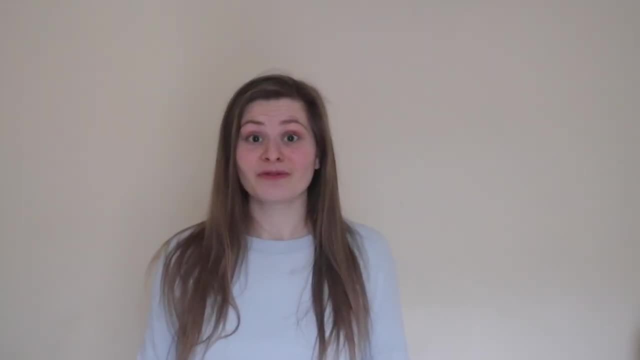 to give three reasons, but remember, if you do know any more, you can show off how much you listened in the videos by writing as many as you can think of. Now you know what you've got to do. you're going to pick an animal, create a fact file about them and tell me what you've learned about. 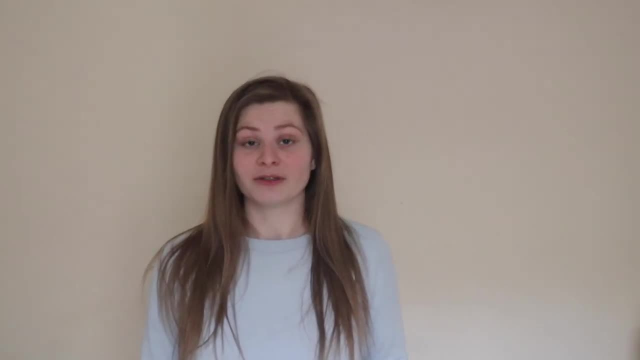 deforestation. Now I'd like you to go and watch a couple of videos on deforestation to help you understand this term a little bit more. then I'd like you to get stuck into the activity. Bye, everybody. 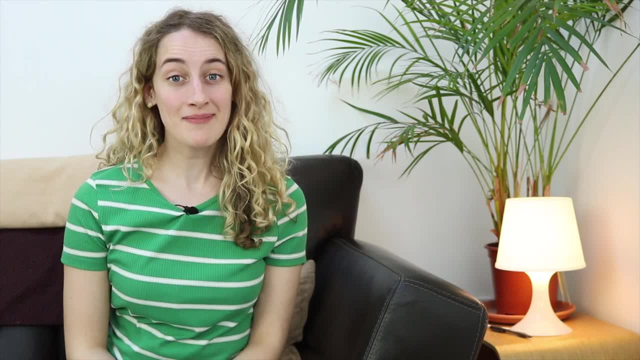 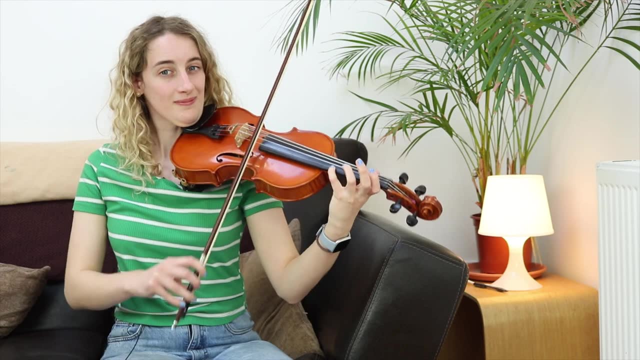 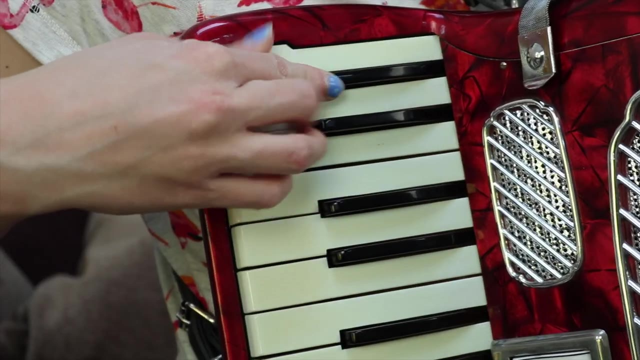 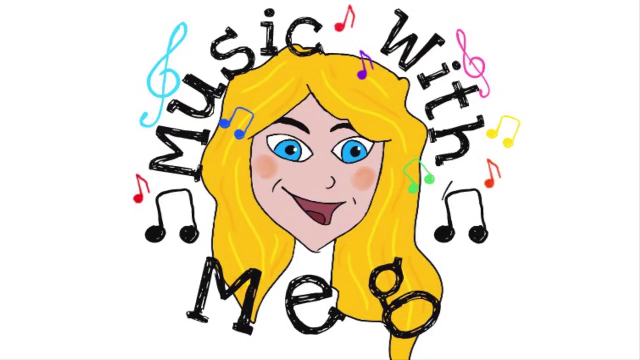 Hi everybody and welcome to Music with Meg. I'm Meg and I'm here to introduce you to the wonderful world of music. Have some fun. Music with Meg. It's time to sing along. Music with Meg Instruments. Will we meet? What will we learn about this week? Everybody follow me. It's Music with Meg. 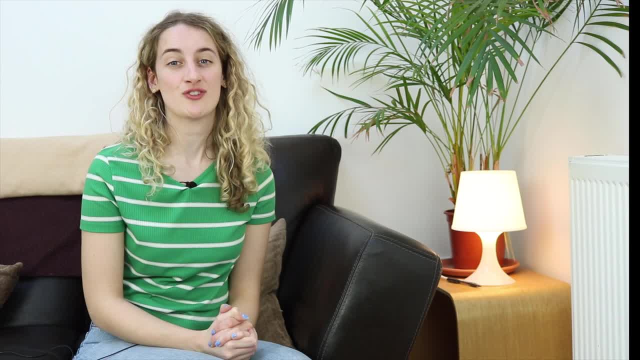 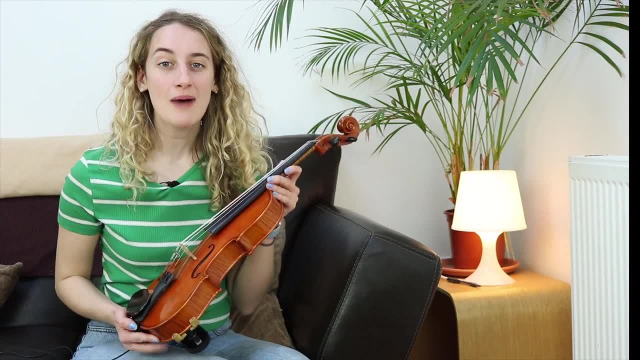 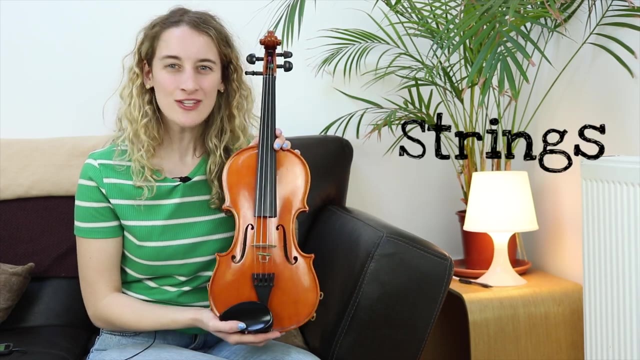 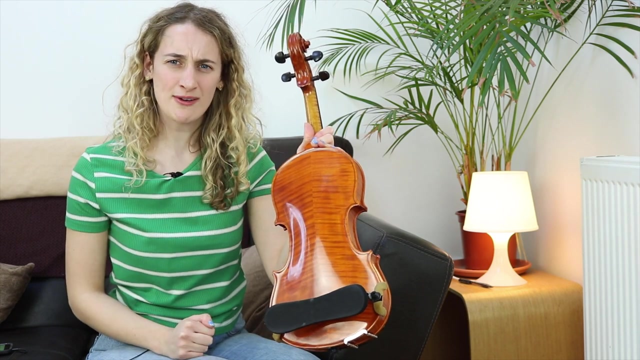 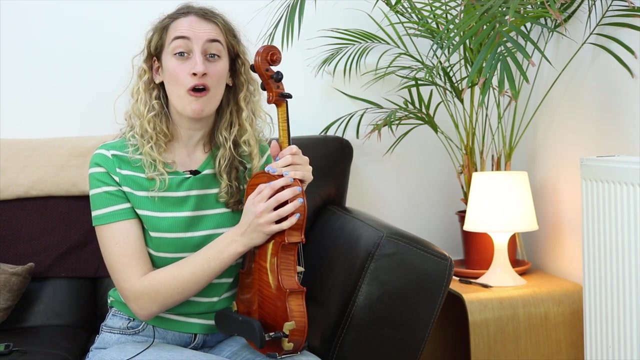 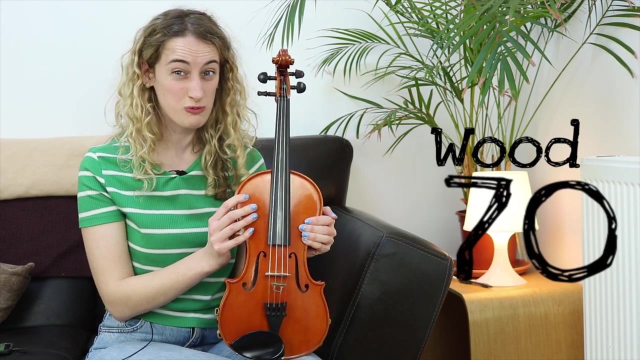 Every week, I'm going to introduce you to a new instrument, So let's see what instrument we've got to meet today. This is my Meg Violin. My violin is a member of the strings family, And can you guess what my violin is made of? Let's have a listen. What material is that? That's right, My violin is made of wood. In fact, my violin is made of 70 different pieces of wood. Now let's take a closer look. 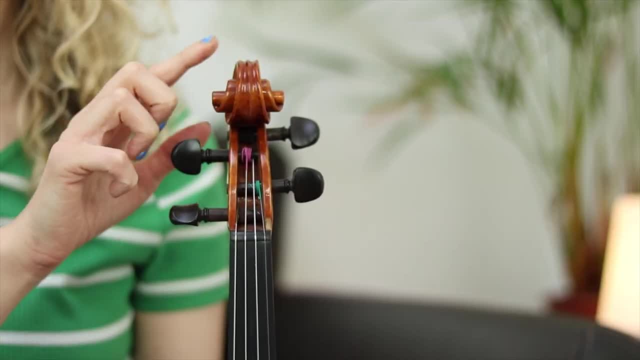 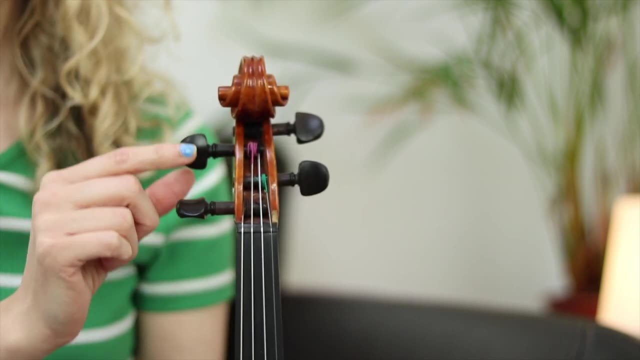 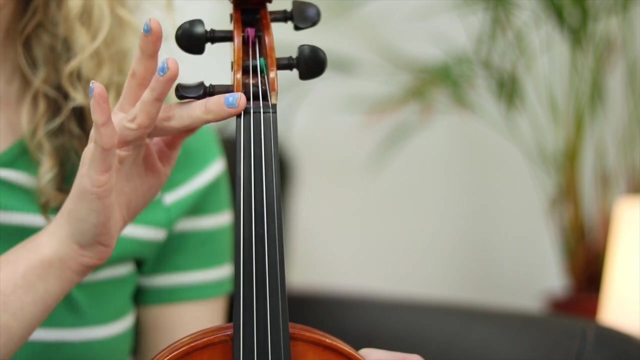 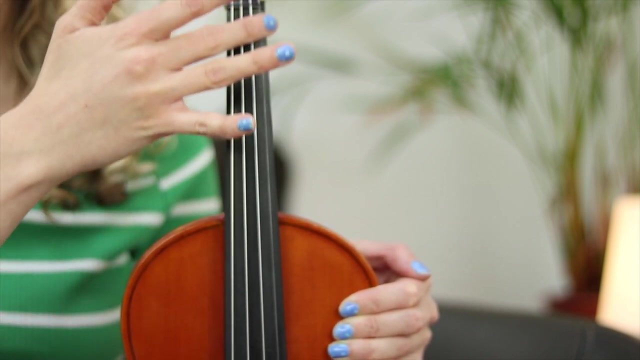 This is my Meg, A large scale. Let's take a closer look at the different parts: how I make my violinז. The top of my violin is called the scroll, And below that we have the pegs which we use to tune my violin. We need to tune to make sure that we are all playing the same notes. Just like you, my violin has I neck And on top of my violin's neck is a long black fingerboard which we use to change the note. Below that we have the wooden bridge And I'm playing the note by Just taking the books.